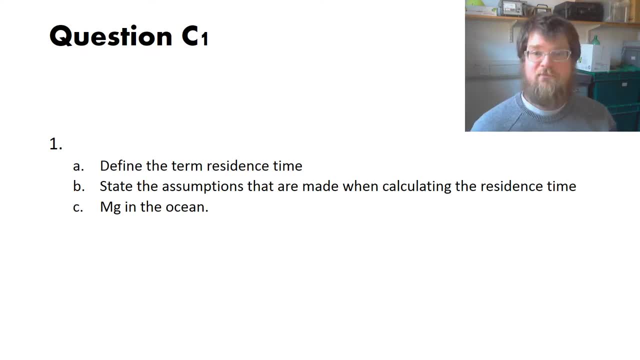 And we'll go through that in a bit and then state the assumptions. Okay, This question clearly had two parts to it. Quite a lot of people missed out on full marks, or at least a large portion of the marks, through not answering both of those parts of the question. 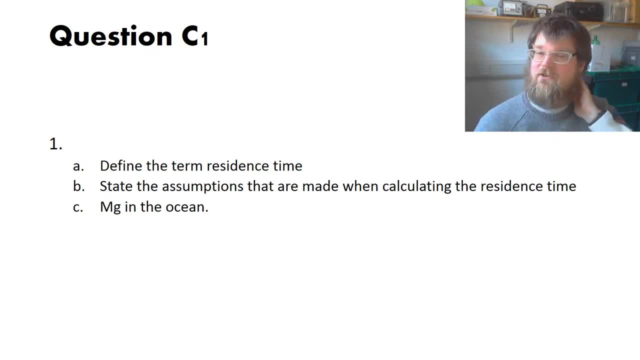 And then the last part I put in. this part I'll see here, which is not really a separate part of the question. but the question asks about calculating the residence time of magnesium in the ocean. So if you're going to use any examples in your answer, those should be from the magnesium cycle in the ocean. 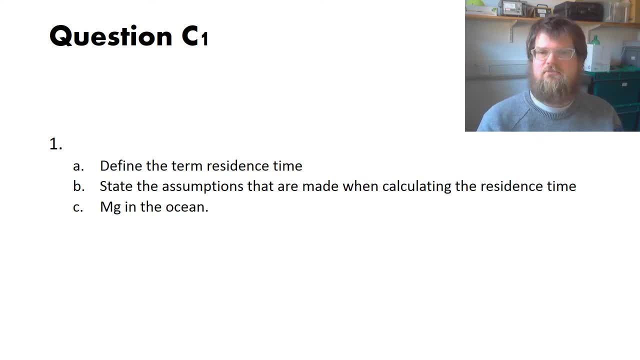 So what are the fluxes in from magnesium? Where does the magnesium come into the ocean? How is that relevant to measuring the residence time, Those kind of details to get the top end of the mark scale? So what is residence time? So these are some slides from the lectures. 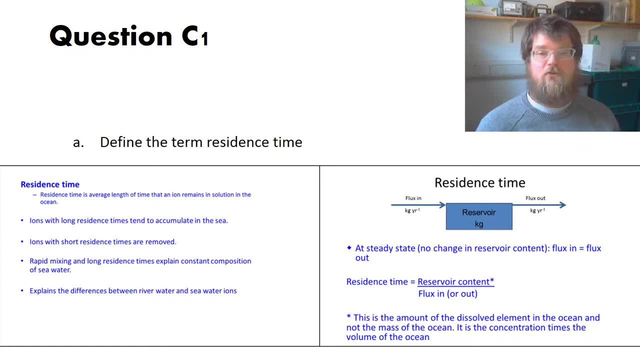 Which you should know and love. So I guess first of all there's a kind of a words definition of residence time. That's over here. So the residence time is the average length of time that an iron, any one particular iron of that substance is present in that reservoir. 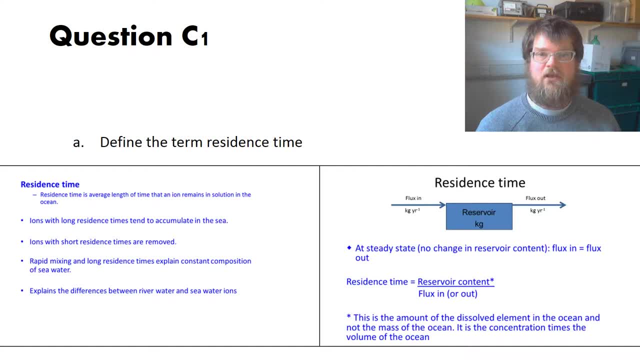 Okay, So an example of the ocean. it's like how long is an atom of magnesium in the ocean on average from when it enters in the flux in to when it's removed? So you can express that as a an equation, which quite a lot of you did, which is pretty good. 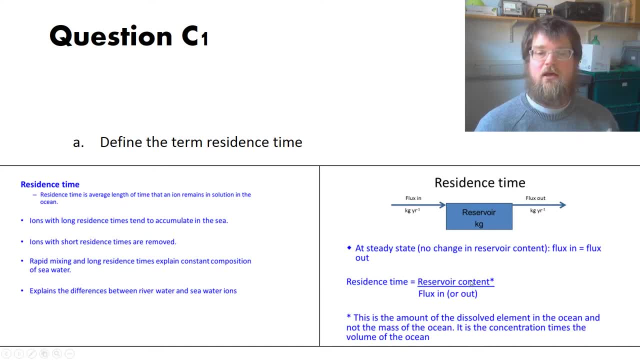 The residence time can be calculated by measuring the total content of magnesium in the ocean and dividing them by that, by the flux in or the flux out. So important here that the what we mean by reservoir content, this is not the size of the reservoir. 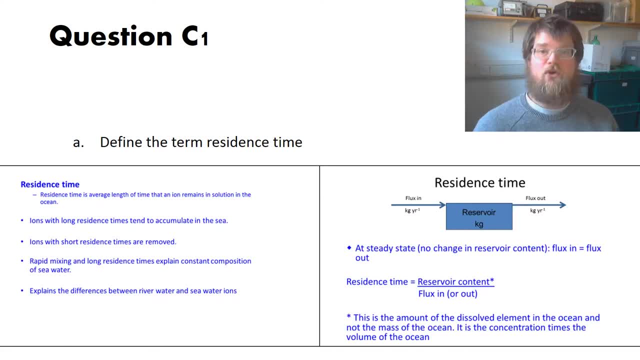 It's the amount of magnesium in the reservoir. It doesn't matter how big the ocean is, It's how much magnesium is in the ocean And similarly, moving on to the assumptions that go into this. So I think many of you mentioned that we have to have the flux in equal to the flux out, so that this flux in has to be the same as the flux out. 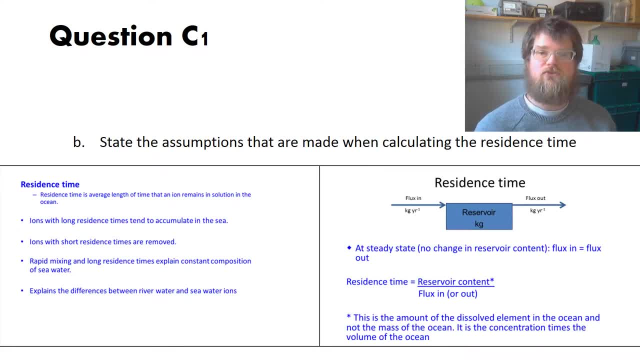 That therefore implies that there is no change in the concentration of magnesium in the ocean at the time it's being measured, So We call a steady state. That would also be an important thing to mention. Other people, or some people, also went on to mention things about knowing all of the fluxes. 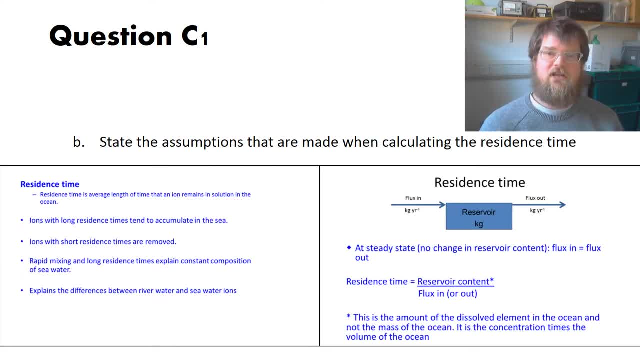 Okay, And that's also quite important, especially with magnesium, because some of the fluxes are at the sea floor, either through hydrothermal activity or incorporation in clays and stuff at the sea floor removal fluxes. So getting a good measurement of those may rely on some assumptions. 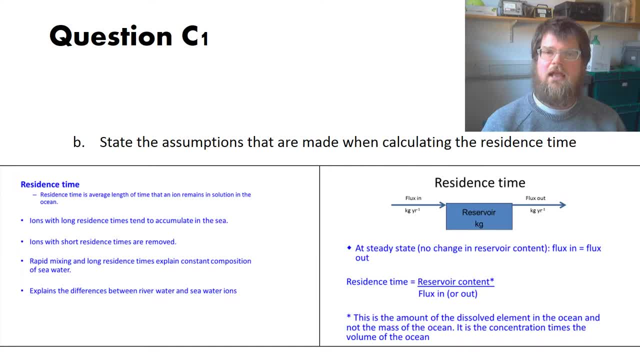 So assuming that we know what all of the fluxes are And they are well represented by our measurements, is also an important thing to include in a full answer for this question. Okay, So where did where did people go wrong on this? This question? 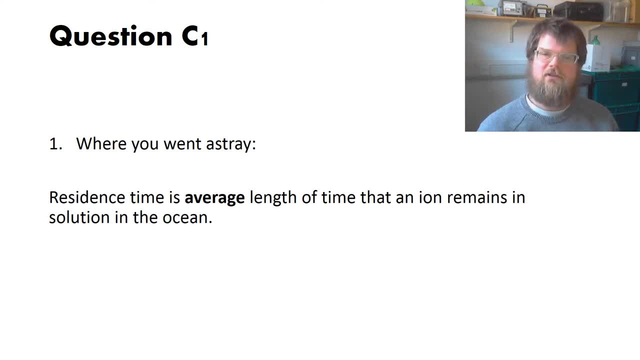 So I guess almost everyone who wrote down the description of the definition missed out the word average. Okay, So it's the average amount of time that an ion of that particular element is in the ocean. Only lost a few marks for that. But. 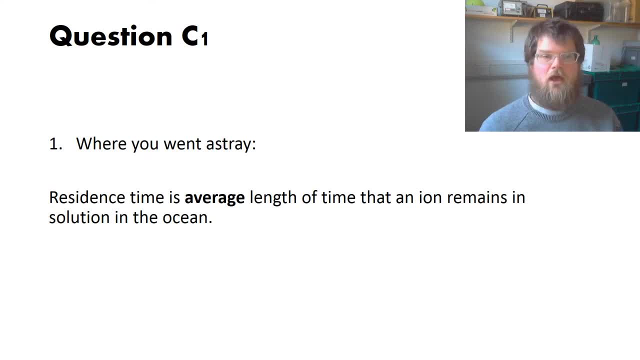 Still, you know why be wrong when you can be right. Quite a lot of you that wrote down the. the equation form of the definition confused the reservoir content with the reservoir size. It wasn't clear in your answer. even though you might have meant the amount of magnesium, it wasn't clear that you didn't mean the amount of ocean. 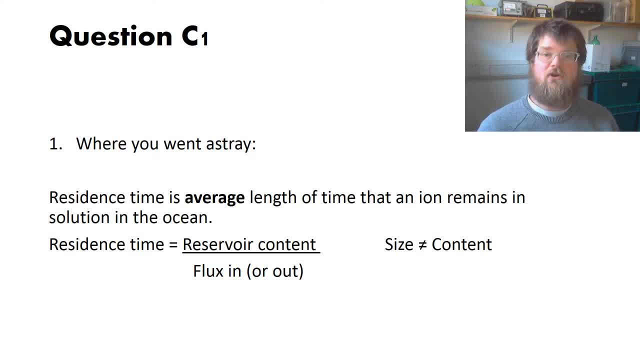 So it's really important to make clear in your answer that the reservoir content is the amount of magnesium. So it's really important to make clear in your answer that the amount of magnesium is the amount of the concentration times the volume. But yes, that's just a little thing that people got wrong. 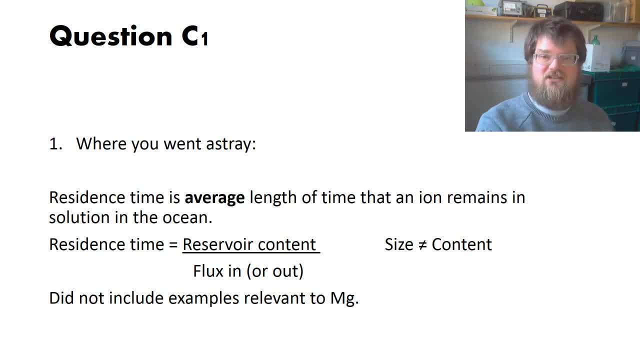 And then I think the thing that most people didn't get the full marks, they didn't really use examples from the magnetic cycle to expand and demonstrate their art. So there's a There's the first question, which was some, was mostly, mostly answered. 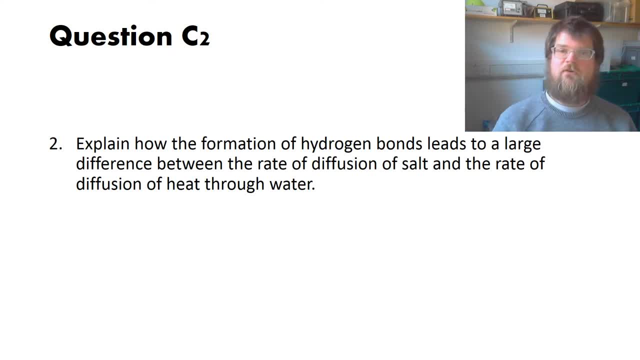 Well, which was nice. Okay. So moving onto the second question. So there's this. this question down there. Okay, So this question down there. question: So: explain how the formation of hydrogen bonds leads to a large difference between the rate of diffusion of salt and the rate of diffusion of heat through water. 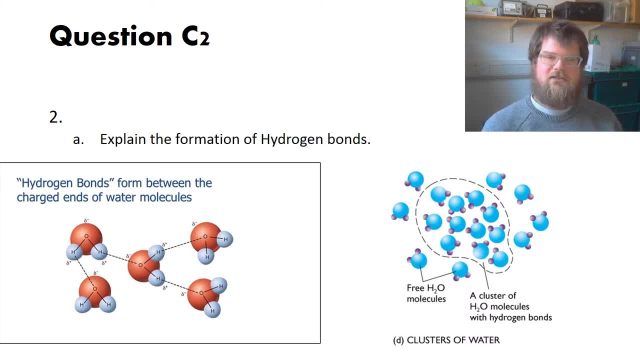 So again, breaking this up into kind of like mini parts that really explain the formation of hydrogen bonds and then move on from there to talk about diffusion and how hydrogen bonds then affect diffusion. The first part here explain the formation of hydrogen bonds, I think quite a lot. 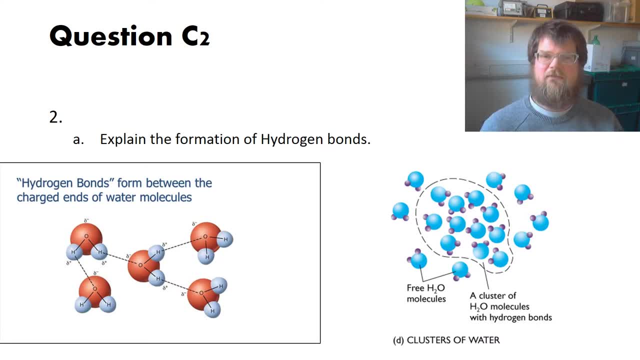 of people did a reasonably good job of this. There was a little bit of confusion in some places about exactly where the hydrogen bond is. a few people had it between the oxygen, let's say between the oxygen and the hydrogen. that's not the hydrogen, The hydrogen bond is. 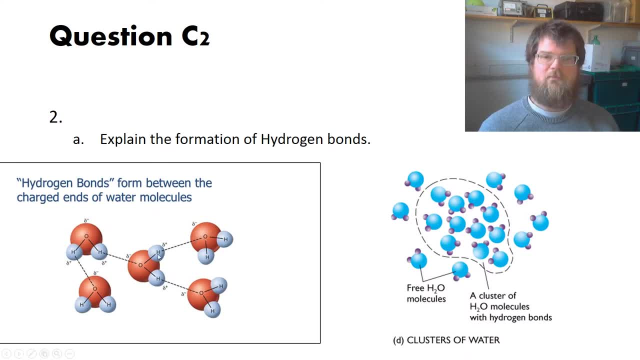 between these polar molecules, so between the polar ends of the of the water, between a negatively kind of small negative charge in the oxygens and small positive charge on the hydrogens. Those are ionically attached together, electrostatically attached together, forming the hydrogen bonds. 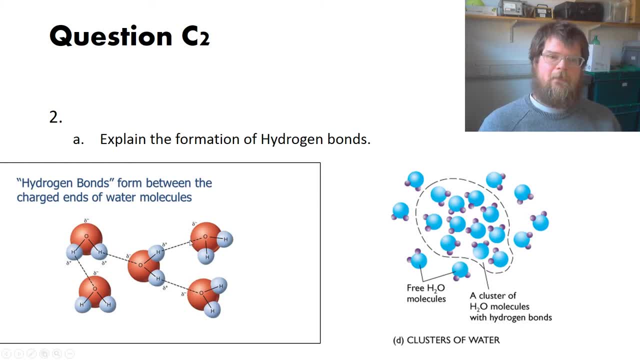 these, uh, quite strong intermolecular bonds. okay, so explaining the formation of hydrogen bonds, that's part of the answer, um, also mentioning that how that affects the structure of water, because that's relevant then to the next part of the question, which is really on fusion. is that, uh, in water? 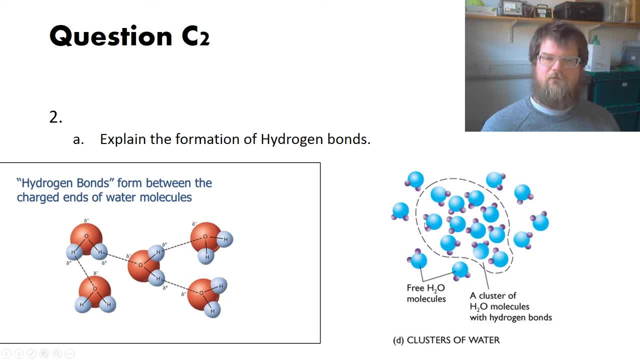 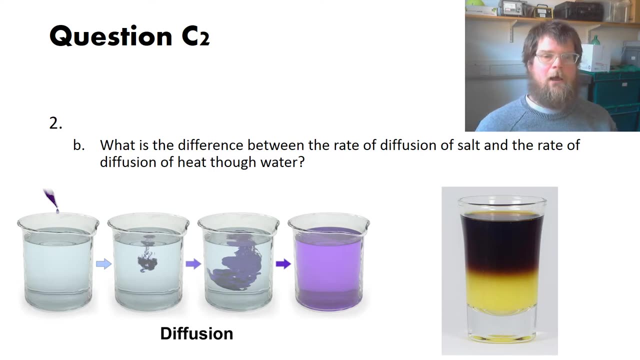 these, these, these hydrogen bonds tend to form kind of clusters of water molecules, kind of clumps of water, that kind of that act as a whole rather than as completely free, individual molecules of water. um, yeah, um. so i guess the next part of the question really needs you to know, uh, what the 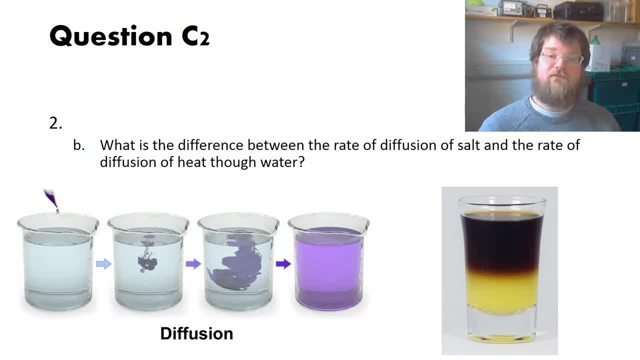 difference is between the rate of diffusion and the rate of rate of diffusion of salt and the rate of diffusion of heat. so before you can say how um hydrogen bonds affects this difference in rates, you need to know which one is faster um. so looking back through the lecture notes, i realized that i i used this: 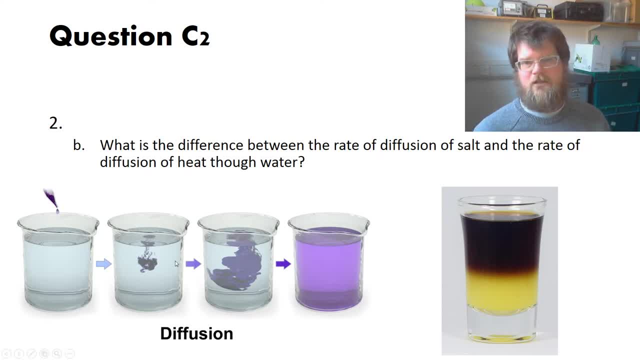 this image over here, um, which was the um, uh in the what is diffusion side, and it's slightly misleading here because this this shows kind of like a drop of dye being added to some beaker of water and you can see that all these plumes and swirls of water and gradually the the dye gets. 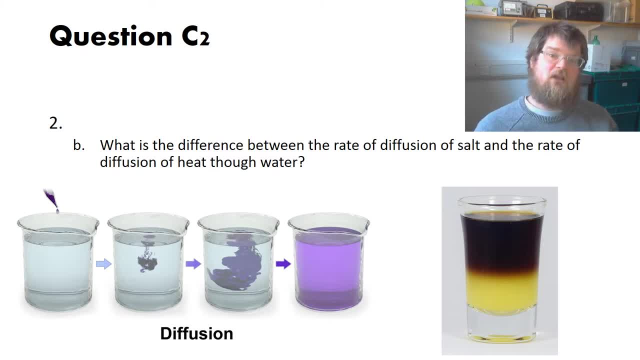 spread out, so that's spreading out of of the dye is could be um due to diffusion. but what isn't diffusion is these, these swirls and these mixes. this is convective um diffusion and this is because the water is moving around and acting to physically stir up, uh, the solution and mix out the um concentration of dye. so, um, really, what diffusion? 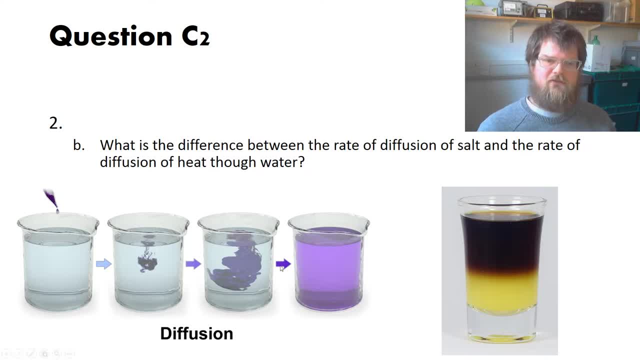 is is is the very, very slow movement of the dye from this plume uh, out into the dye on the out into the water either side of it. so it's not the physical mixing, it's the um slow diffusion or slow movement of these dye molecules through the water. 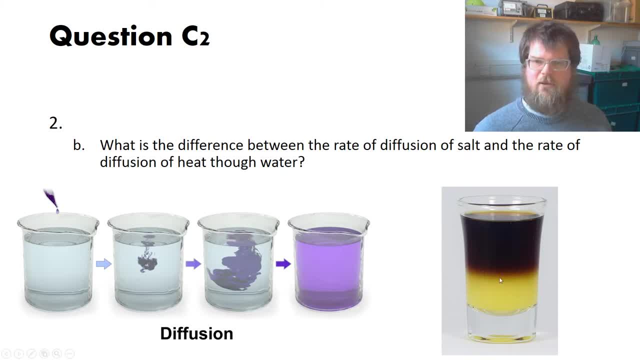 and that's uh, that's kind of quite nicely illustrated here. i can't remember the name of this cocktail, which i've um downloaded on the internet, but you can see this. there's basically this, this blurry boundary between the two layers of delicious beverage, i assume. i think this is. 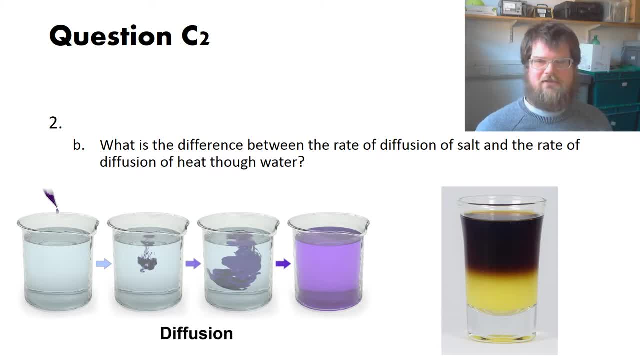 kind of jägermeister and orange juice. i think it has a name, but i'm sure it's disgusting. um, but you can see the uh, this, this, this blurry boundary, this is a diffusion from. this is kind of the jägermeister diffusing into the orange juice. 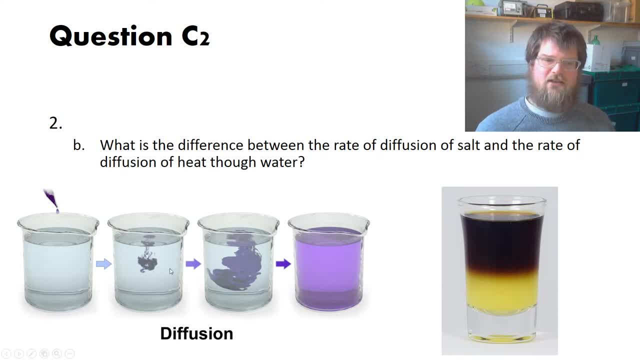 and vice versa. you can see, it's a very different kind of form of than this kind of um physical mixing approach, physical mixing um phenomenon anyway. so we're looking at: uh, what are the the rates? which is basically before we can ask the question. we need to know which is faster, is it? 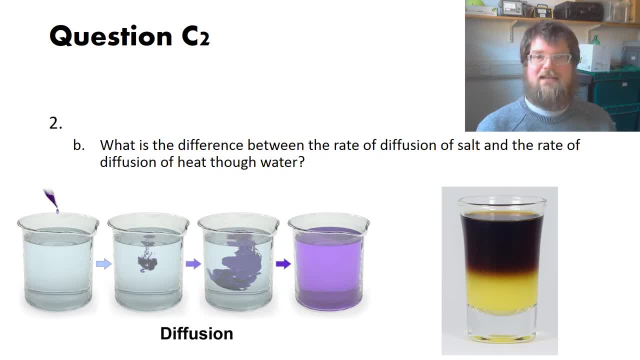 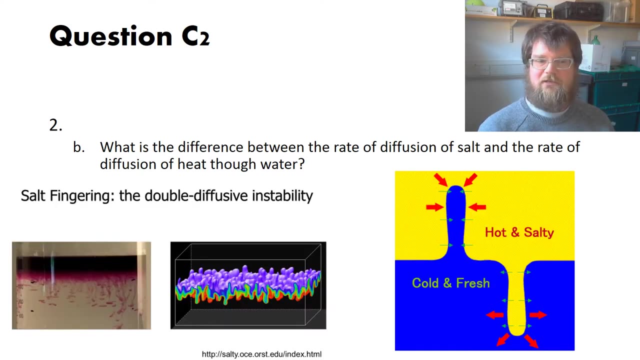 salts diffusion or is it heat? um, and it's heat diffusion, heat diffusion, heat diffuses almost 100 times faster than salts through um, uh, through water. so a few of you got that wrong, um, so therefore made answering the last part of the question more difficult. um, and we can see evidence. 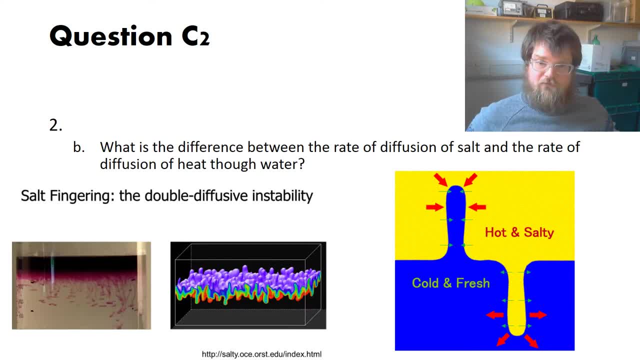 from this, these different uh rates of diffusion, in this phenomenon called salt fingering, which a few of you kind of mentioned in your answer, was great. i mean it wasn't necessary but it was a good thing to add in um, so we can see here that the the heat can diffuse through um, the. 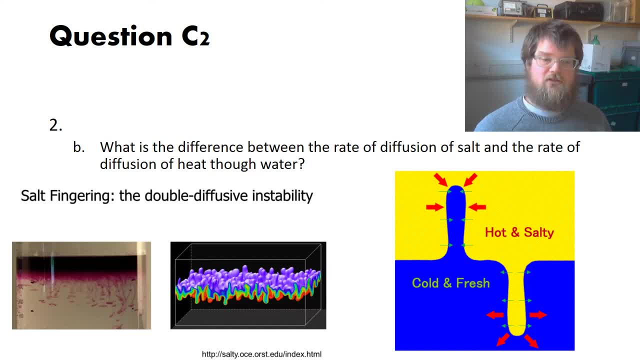 the liquid a lot faster, the water a lot faster than salts, um, and that's what's, uh, that's what's happening over here, in these kind of fingers of of cold salty water that are emerging down from this layer of warm salty water on top. and that's because, if we look at this close-up, schematic- 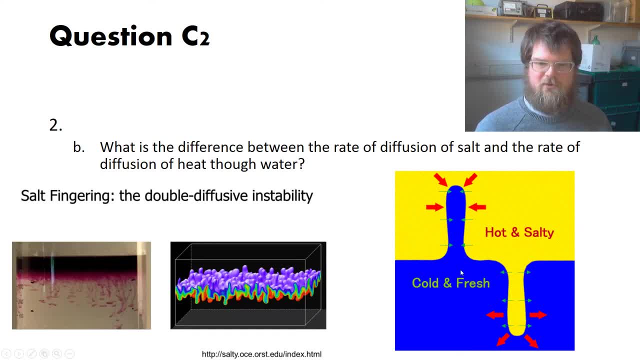 diagram. if we have a kind of any uh disturbance on the boundary between the two layers, uh, heat will diffuse out of the the top layer into the layer underneath. that will happen very quickly, whereas the salt will diffuse much more slowly and that leaves this piece of water here warmer but not salty uh compared to the water um down. 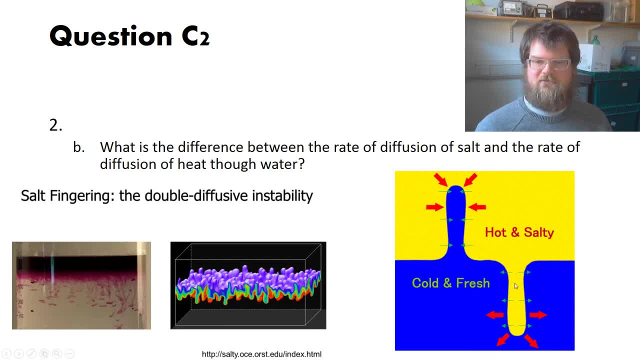 here, so it leads it to rise up and consequently this, this piece of water here which has got lots of heat, which had lots of heat in it, but that's diffused out into the surrounding water, but it's kept its salt, so that's cold and salty now, so that sinks, um so 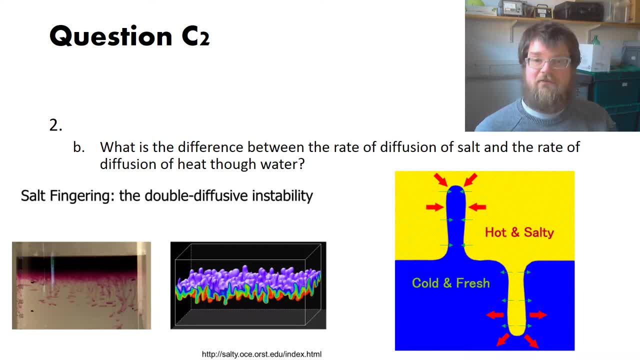 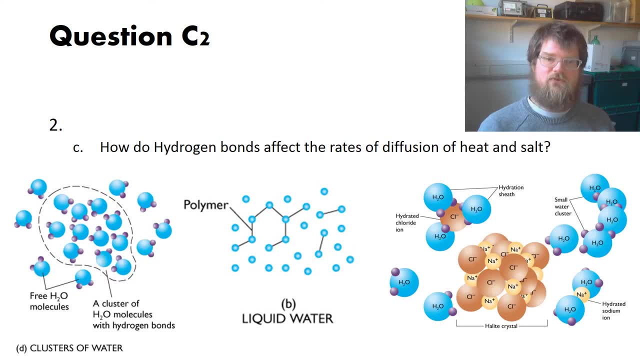 that detail of the explanation. it would be nice to have the answer, but it's not essential. the essential parts really are: how do the hydrogen bonds affect those different rates of diffusion? so heat can diffuse very quickly compared to salt, which diffuses relatively slowly, and the reason for that is: 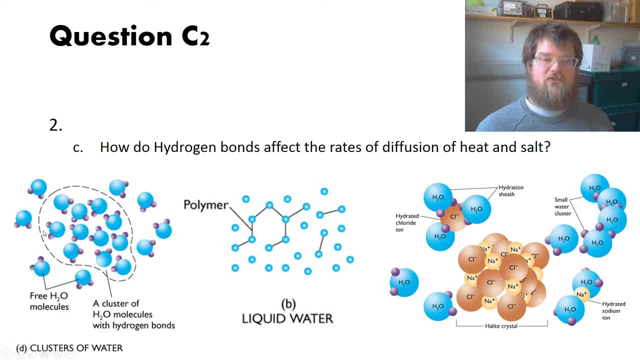 these clusters of water that we have. so if you want to get heat from one side of this cluster to the other side of the cluster, you want to diffuse that heat from one side of the container of water to the other, all you need to do is transfer the momentum of these, these, these um. 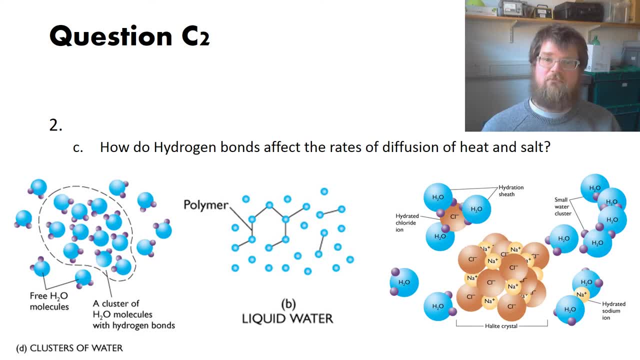 molecules which are vibrating, shaking around because they have some temperature, because they have some heat um contained within them that's reflected in their kind of vibrational energy. and to do that, all you need to do is you start shaking this guy here. that'll, that'll lock into. 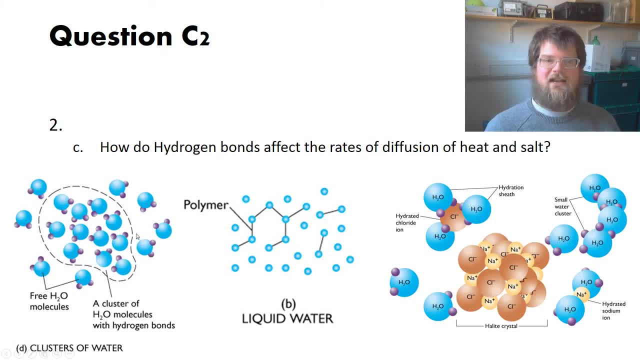 this one, uh, which will transfer that momentum through that cluster of water and actually by bonding together the individual atoms or the individual molecules- sorry, that helps transfer that momentum through that cluster. so that means that heat can diffuse very, very quickly. You physically need to get from one side. your salt has to get past all of these water molecules wiggling its way through and to pop out the other side. 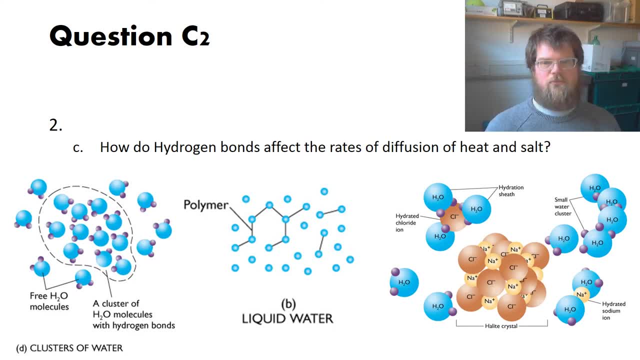 So its concentration can be equalized across the whole body of water. And that's made doubly hard because when salts dissolve in water we tend to have this phenomenon called hydration, where the ions are surrounded by water molecules to kind of neutralize their charge. 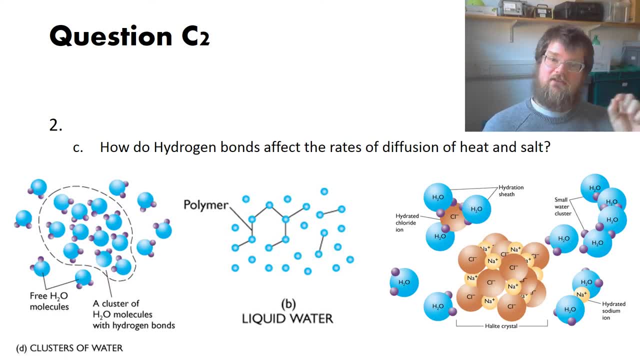 And that effectively makes them even bigger. So you've got to not only get the salt ion to diffuse through all of these clusters of water molecules, you've also got to get all of this baggage that's attached to it, all these other molecules of water which are attached. 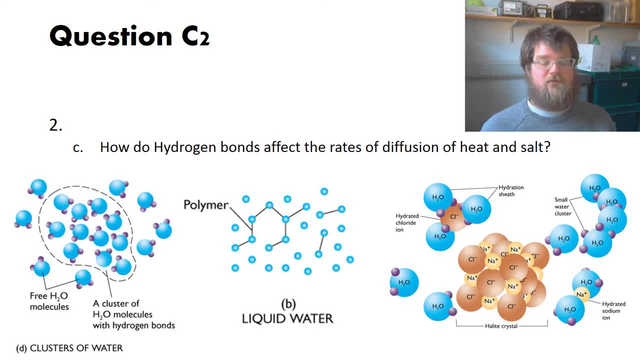 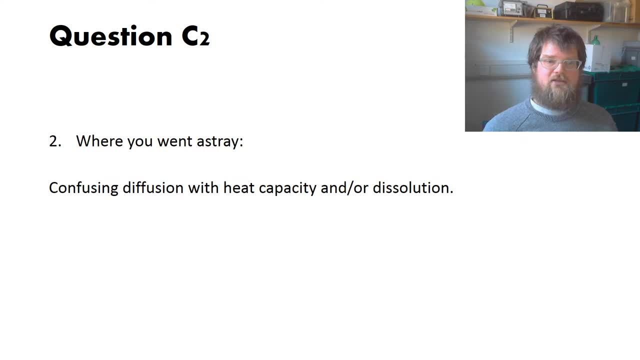 So that makes it even harder to get through. So that's why salt diffuses very slowly. So a few pointers of where people went a little bit astray on this. So one of the really common errors was people actually quite correctly identified that water has a very high heat capacity because of hydrogen bonds, which is correct. 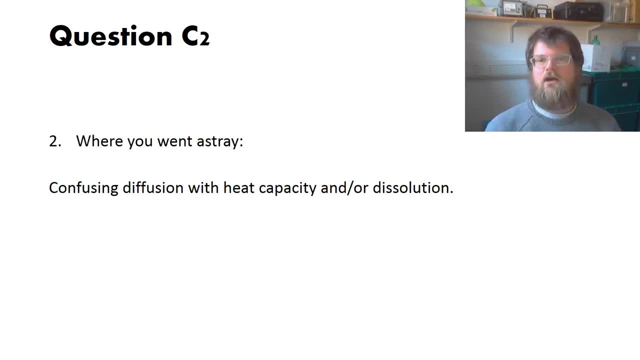 And they identified that water is really good at dissolving ionic salts because of the hydrogen bonds. also correct, But those are the things that are really important. Those are not why the rates of diffusion are different. Those are just other properties of water. 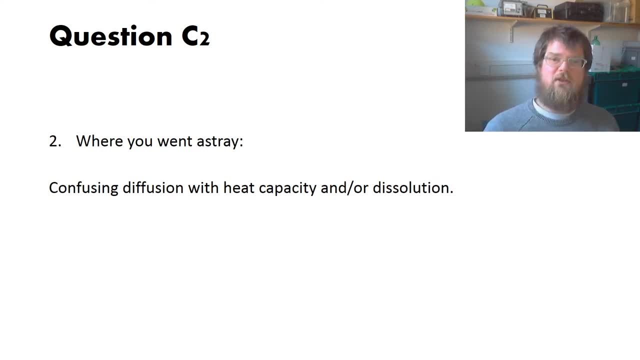 So they were correct, but they weren't answering the question, And this was a common theme through all of the questions in my part of the exam. Quite a lot of people did not specifically answer the question, which is why they got fewer marks. 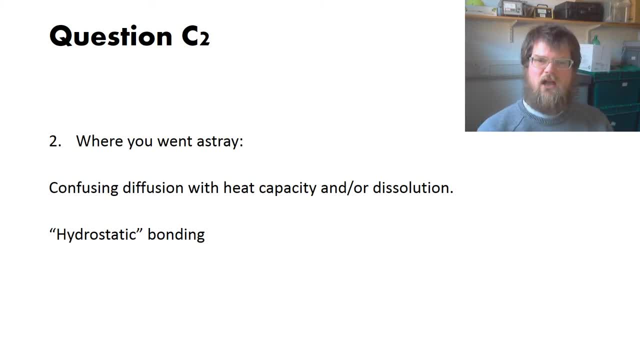 Not less fewer. A few people used the term hydrostatic bonding, which is not a thing. Don't use that, because it's nothing. It's just not a thing. That's incorrect, And quite a few people went through all of the details of describing that hydration of salt ions and how ions get plucked out of salt crystals and stay dissolved, which was great. 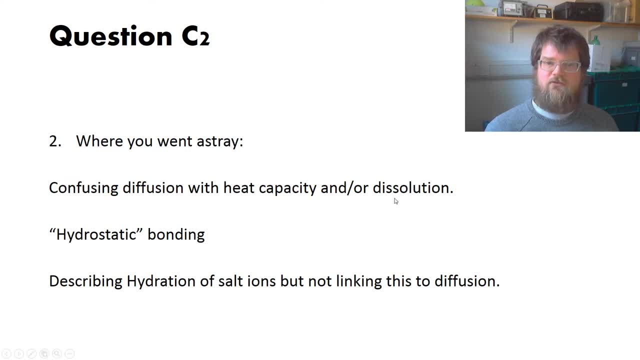 That was slightly confusing, the dissolution with diffusion kind of aspect. Quite a few people did that, But even the people who didn't, they kind of didn't really explain why this hydration of salt ions affected diffusion, Which would have linked it back to the question. 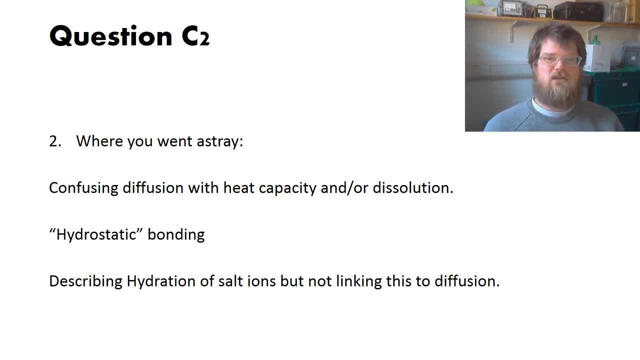 So what you wrote was correct. It just wasn't answering the question, which is what you need to do to get marks and prizes and all kinds of fun things. But again, quite a lot of people expanded on their answer by mentioning the salt fingering thing which I demonstrated in the lectures. 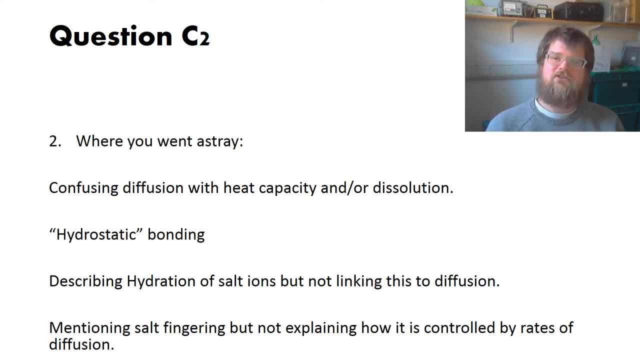 But you didn't really explain how that related to different rates of diffusion. OK, so you didn't go through that. That explanation of how it worked, which would have, would have been better than not explaining, Right? So moving on now to the optional questions. 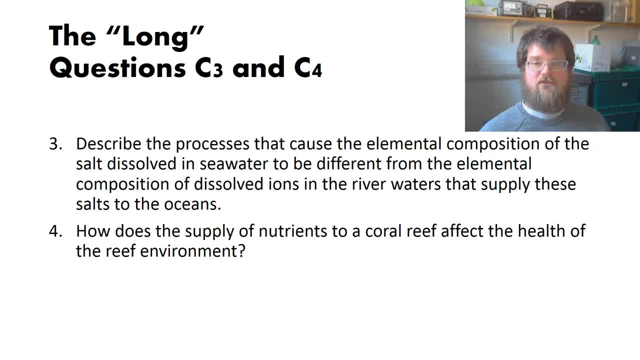 So you had to answer one of these two questions, part C3 or C4.. So the first one was really about sea salts and why the composition of sea salt is different to the composition of river water. Not very many people answer that question, possibly because I went over the last question. 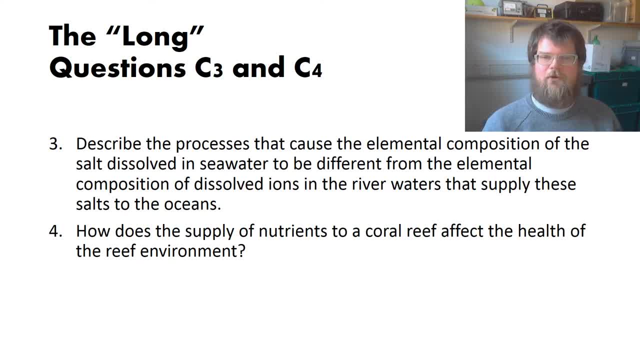 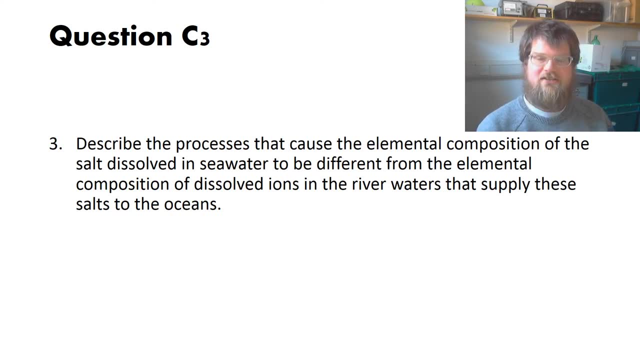 Which was about coral reefs in the revision session. Who'd have thought I would have had an impact on what you answered in the exam? But anyway, I'm going to go through the third one first. So the question is: describe processes that cause the elemental composition of salt in sea water to be different from the elemental composition of dissolved ions in the river water that supply those salts to the oceans? 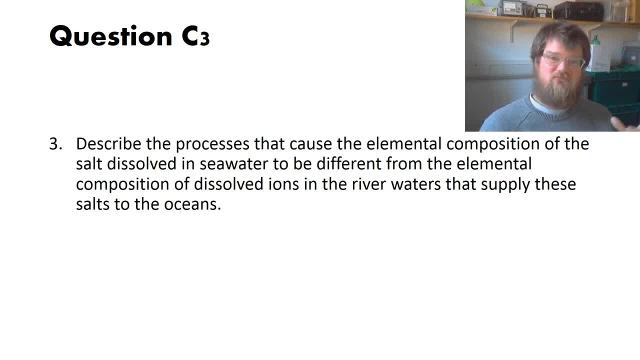 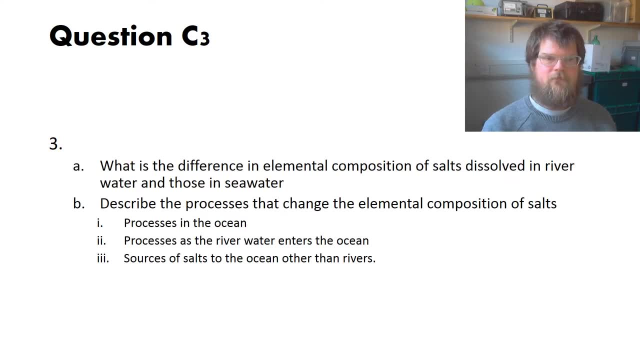 So quite a lot of words there, But it's really, why is salt in sea water different from the dissolved ions in rivers? OK, so again we could break that up into kind of little mini parts And really, before we start saying, what is the difference, why is there a difference? 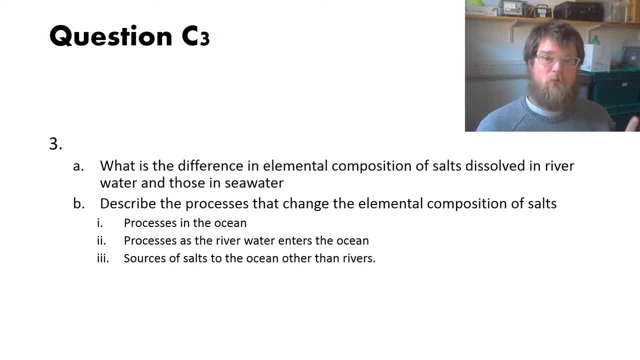 We could really say what is the difference. So not many, many people went into this, But it's kind of implicit in the question that you need to do. It's implicit in the question that you need to demonstrate that the two things are different. 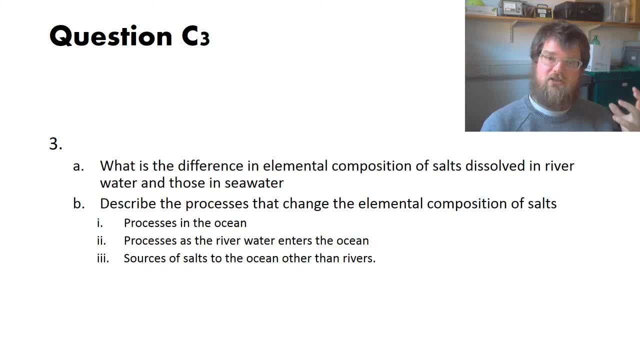 So, first of all, what is the actual difference in the salt composition in sea water versus the salt composition in rivers? And then, once you know that, once you've demonstrated that you know that- I'm sure you all know that, Then you can just start to describe some of the processes, whether they're in the ocean or the interface between the rivers and the ocean. 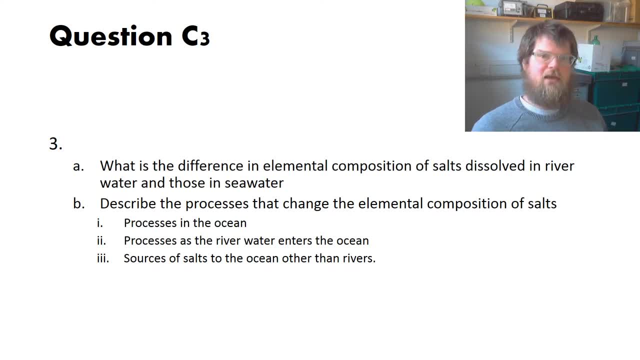 Or are there other reasons, other than processes in the ocean, that the salt compositions might be different? There are different sources of salt in the oceans. Not all salts come into the ocean in rivers. So this is an opportunity for you to kind of expand and kind of like take the question a little bit further. 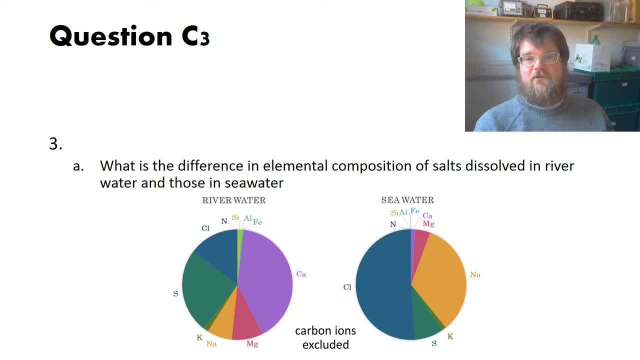 So, first of all, the difference in the composition of the river water and sea water. So you can see, sea water is mostly made up of sodium chloride, lots of chloride ions, sodium ions, a bit of sulphur, a bit of magnesium. Not really a lot. I mean, there's a lot of other things dissolved, Mostly basically sea salt, sodium, chloride, Whereas river water has a very different composition. It's mostly made up of sulphur and calcium, some more magnesium, very small amounts of sodium compared to the amount of sodium in sea water. 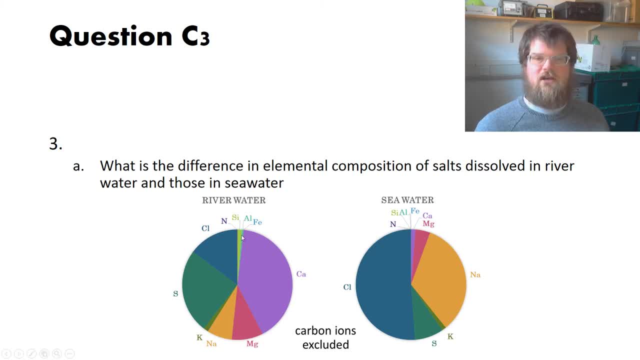 It looks quite a small wedge on this diagram. Silicon is significant in river water. It's almost completely insignificant as a component of salt. Certainly It's very important nutrient if you're a diatom or a sponge, But other than that it's not really. 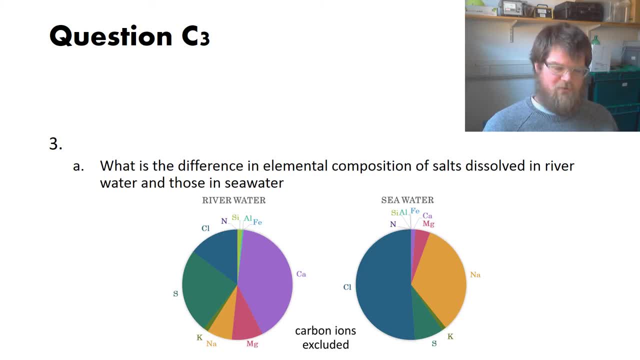 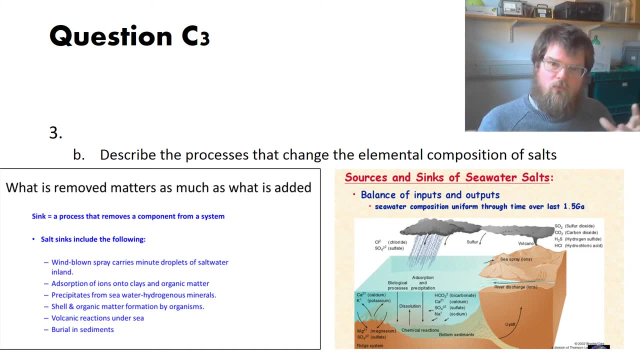 If you dry out some sea water, you're not going to be able to extract huge amounts of silicon from that Anyway. so now we know that they're different, We've got to ask ourselves why they're different, And the difference comes down to the different sources. 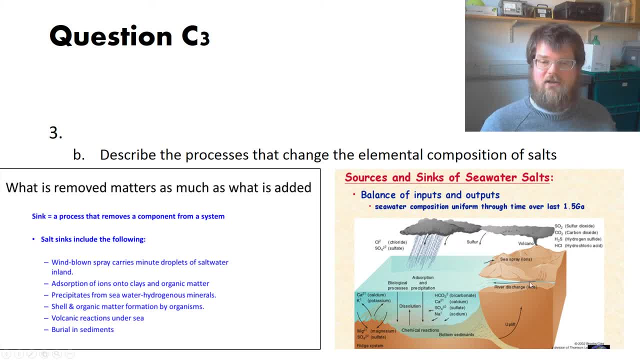 So we might be adding stuff to the ocean by river And that should have the same composition as river water salts, But we're also taking out of the ocean via other processes which might fractionate these salt elements, And we're also potentially adding in elements from different sources. 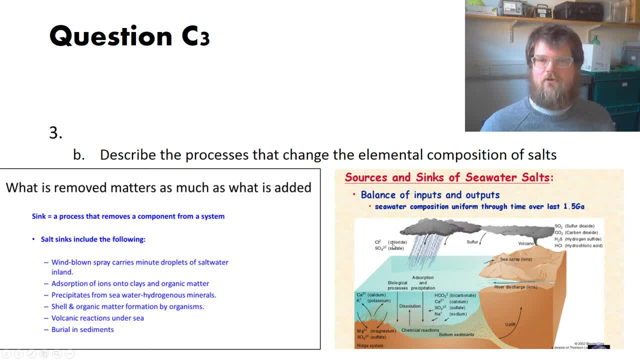 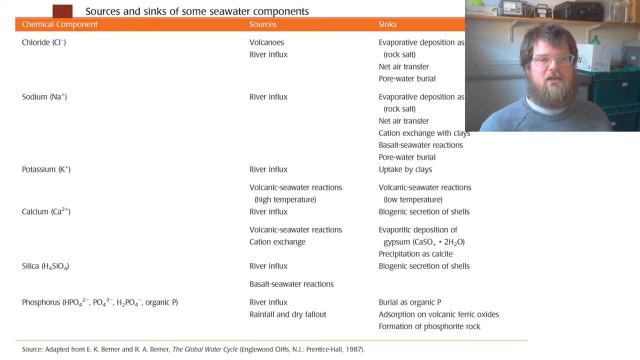 So maybe volcanoes, in the example of chloride, is a different addition method route than rivers. So it's important for you to identify in your answer that the solution to why these things are different is down to sinks as well as sources. Okay, And just to have a look at some of the examples that were in the lecture, you can see here that the removal of elements like chlorine and sodium are processes that are very, very slow. 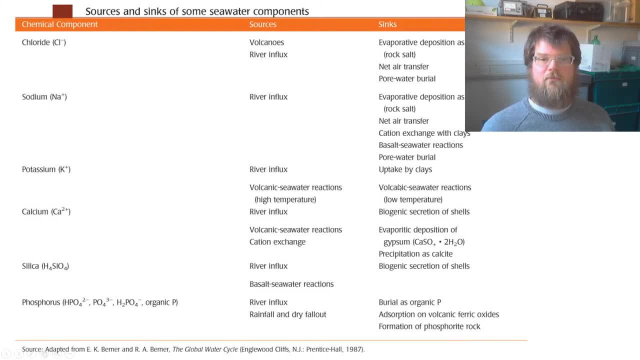 They're low rates of removal. So by either poor water burial, so just water that's in between grains of sediment. as those sediments get effectively subducted in subduction zones, a very slow process Evaporates. So this is kind of the ocean evaporating. 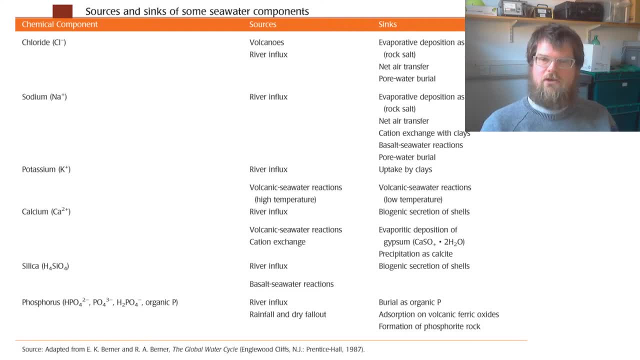 And it's a very important process- locally, in places where it's very hot and small bodies of water isolated. But as far as the whole ocean goes, sea salt's not spontaneously precipitating out, Spontaneously precipitating out everywhere, Whereas other elements, like some of the elements, like calcium and silicon- these elements which are relatively enriched in river water but depleted in ocean water- 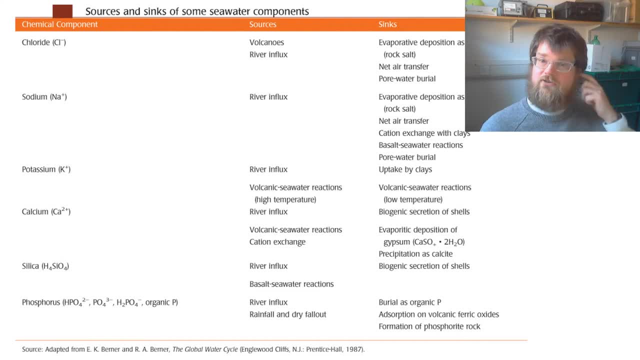 Those are removed by much more rapid processes that have got much higher potential fluxes. So biogenic secretion of shells. If you're a coral reef, you're producing a calcium carbonate skeleton That'll be removing calcium from the ocean. If you're a diatom or a sponge, you'll be producing a test or some spicules that are removing silicon from the ocean and putting that into sediments. 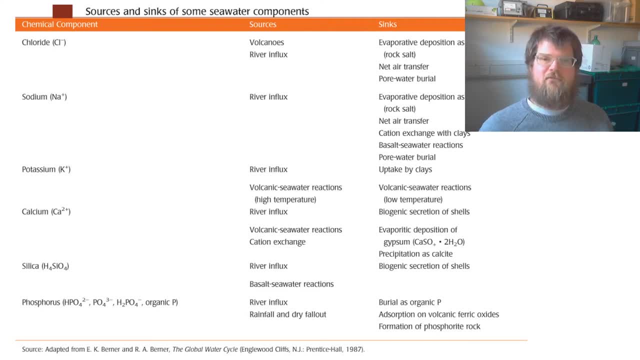 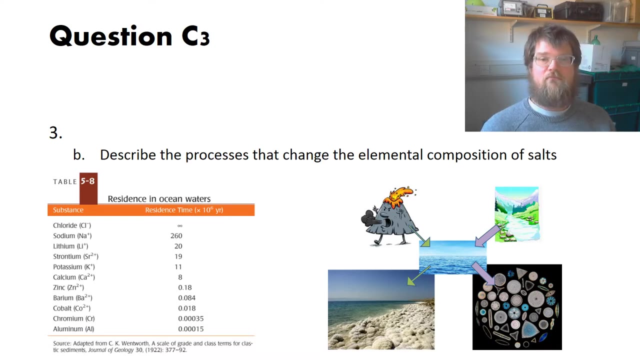 So if you have high rates of removal of an element, then that will lower its relative abundance in sea salt composition. So that can be linked to the residence times. So if you have high rates of removal, If you have high rates of removal of an element, say calcium or silicon, then it will tend to have a lower residence time than elements like sodium or chlorine which have got much slower removal rates. 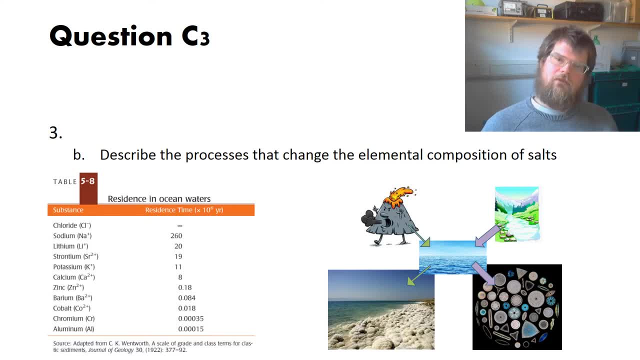 So that then links together the idea that the elements with long residence times are relatively enriched in their concentration compared to river water, Whereas elements with shorter residence times are depleted Well the concentration of other salts compared to those in river water. So I think quite a lot of you who answer this question got kind of most of those details, which is pretty good. 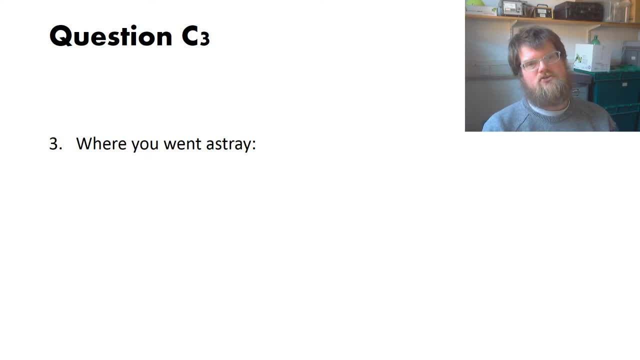 Some of the things where you went astray a little bit, So those that did quite badly on this question really mixed up the idea of changing the composition of the salt, So changing the composition of the salt, So changing the composition of the salt. 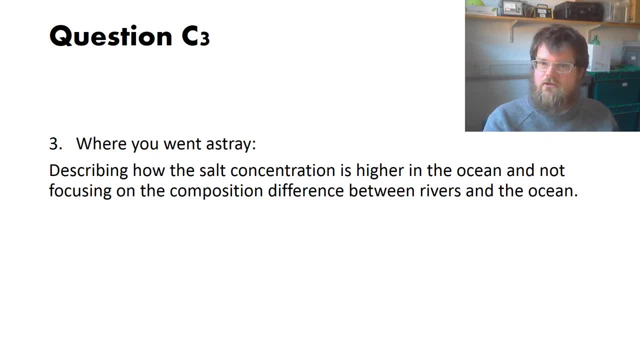 between which elements are the major elements of that particular body of water. So, for example, changing river water, which is mostly calcium and sulfur, to a sea salt, which is mostly sodium and chlorine, with changing the actual concentration to the amount of salt. 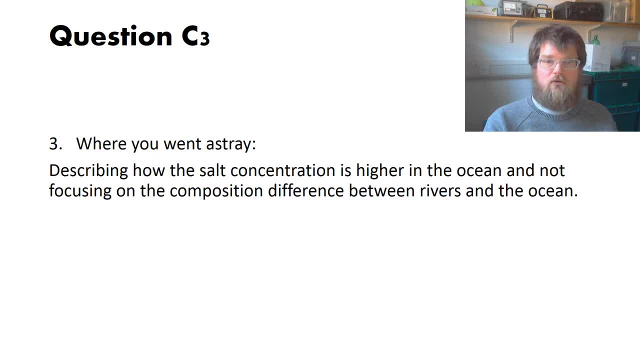 So the ocean is much more salty than the rivers. It has much more calcium and sodium and sulfur, much more everything than river water. That's not what the question was asking. The question was asking about the compositional change, not the concentration change. 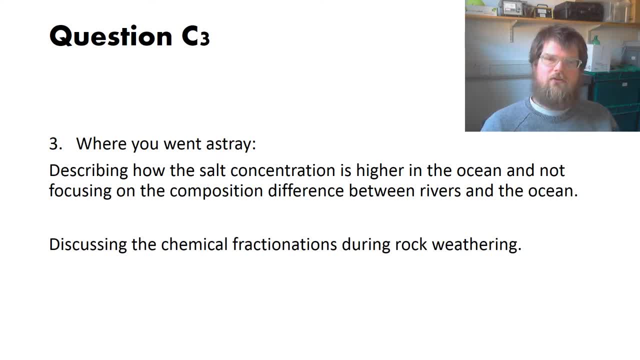 A few people focused in on the difference between the continental crust composition, so rocks and river water. So there is a similar fractionation there to do with also residence times in river water. But the question was asking actually about residence times in and the change of composition from the river water. 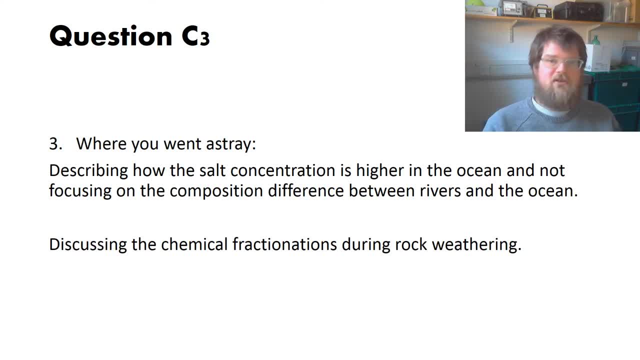 To the ocean, not rocks to river water. I mean, some of the stuff that you wrote down was still correct. It just wasn't focusing on the question which is how you get the marks And another thing that people really missed out on some easy marks and they went through all of the trouble of describing some of these processes of residence times being important and the removal fluxes being important in terms of determination. 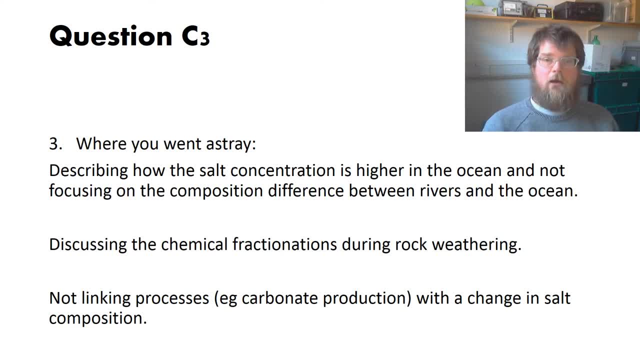 Which elements get enriched, which elements get depleted, but they're not linking that to the final answer of what happens to the relative concentration. So for the example of calcium people- some people it may have been, you probably wasn't, because this question wasn't asked by everyone- said removal of elements by shell formation, but then didn't say 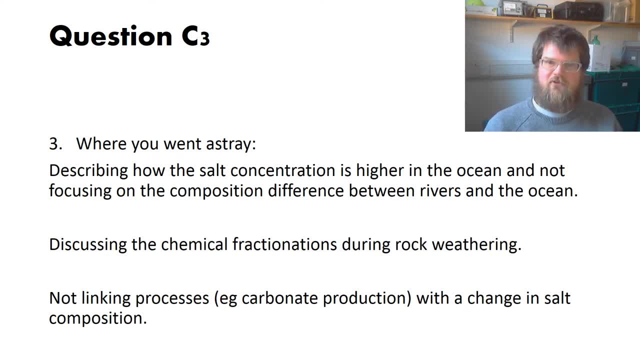 For example calcium, which is then reduced in concentration relative to the other element. because I mean it was, it was a small additional area which would have got you a small additional, small additional addition, additional addition, something you could have added, just a small detail of explanation which would have given more marks. 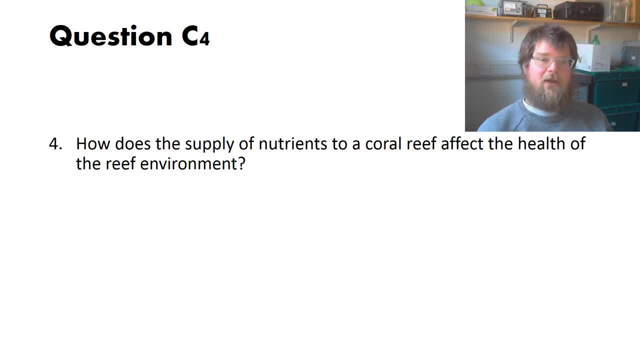 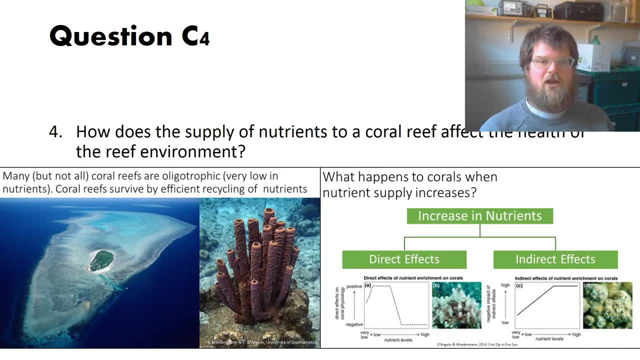 Okay, so the last question, which was, I think, answered by most people: how does the supply of nutrients for reef affect health of that reef? So, really, what we're looking at here is coral reefs. I didn't really specify, but it was a warm water or a cold water, coral reef which is, so I didn't mark you down for that. 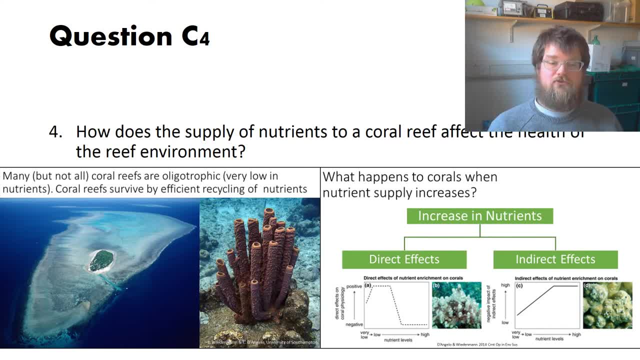 If you went on about cold water coral reefs, which also require nutrients in a different way, But most people wrote about the illogotrophic reef environment, so nutrient, And I guess The answer needed to basically cover quite a lot of the material that's in the second part of the last lecture. 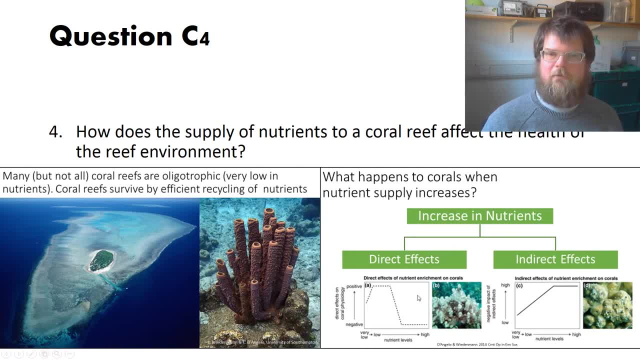 So we're looking at first of all, some, all these coral reefs do need some nutrients, So they they need some, and if you've got no nutrients, give them a little bit of nutrients. they start to behave, or they start to. the environment starts to improve because they can produce more organic matter through their symbiotic zooxanthellae. 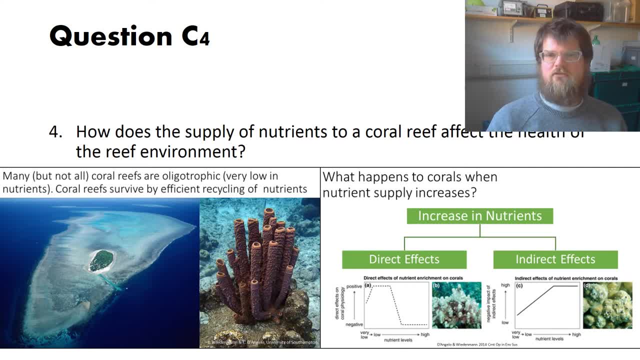 More organic matter can be produced. But if you increase the concentration of nutrients further, then you can have detrimental effects. So a small amount of nutrients are good, but as soon as you start getting lots of nutrients it's bad. And that badness can be either through what we call direct effects or indirect effects. 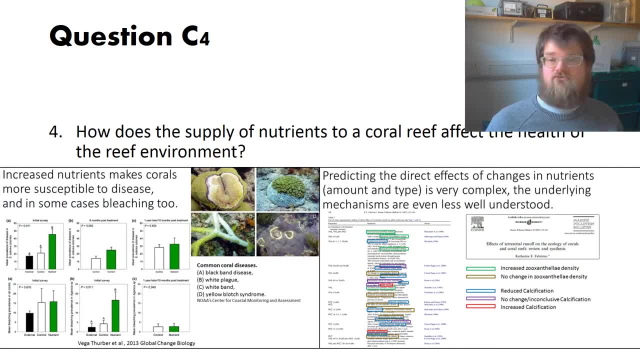 So just looking at the direct effects first, you didn't have to structure your answer particularly about the direct and then do the indirect. I wouldn't really Fussed about the structuring of your pros, but some of the direct effects. I think one of the one of the things that I did give credit for was was noting that these direct effects of nutrients are actually quite poorly understood. 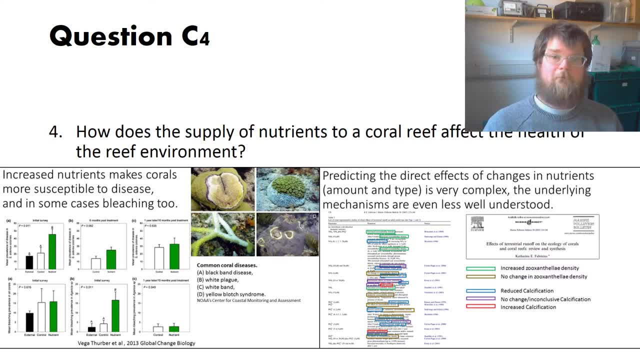 So if you mentioned that, that there is scientific controversy about this, then that was great. And some of these direct effects are that that it changes the, the, the corals susceptibility to disease and bleaching, which was kind of the direct effects. 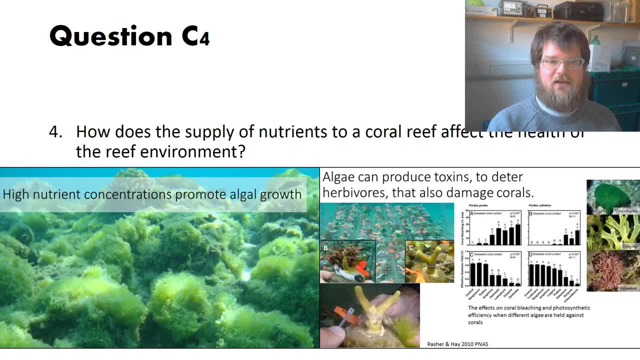 Most of the answer, most of the effects, In fact to surround about these indirect effects when we have algal growth. So if you have lots of nutrients that promotes algal growth, either in the water column or actually on the seafloor, so you get benthic algae and that can have all kinds of impacts. 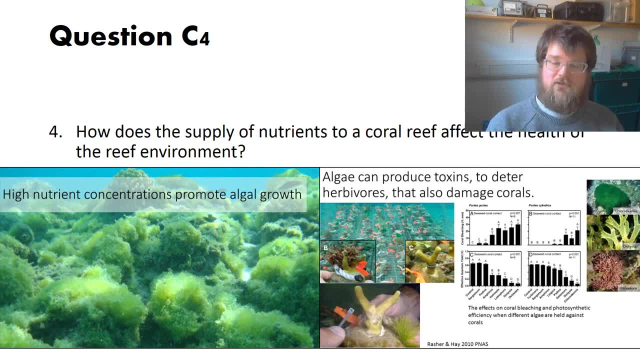 It can lower the light levels. It can kind of physically cover some of the coral. So it can't photosynthesize because it's not seeing any light. Well, the zoo's entirely can't photosynthesize. We also have Some of these benthic algaes, seaweeds. they're toxic. 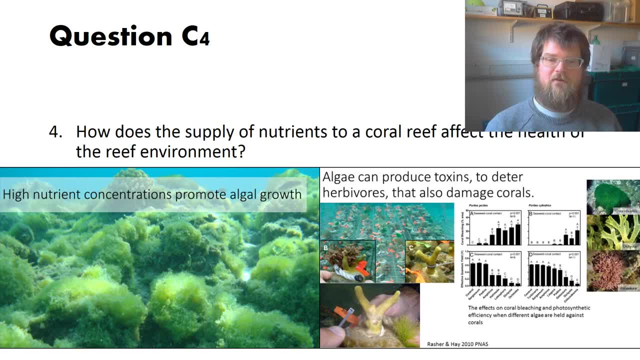 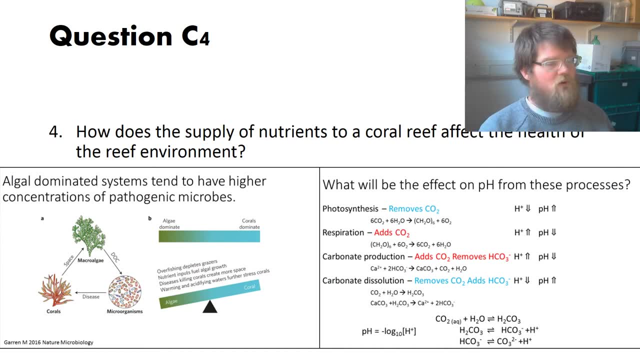 So mentioning that and and referring to maybe some of the details of the stuff here on the slides, that would have been good. If we increase the nutrients and have lots of algae in the water, then there will also be this effect that there's a lot of organic carbon dissolved in the water, as these algae is kind of, they die and get remineralized, break up into dissolved in organic carbon. 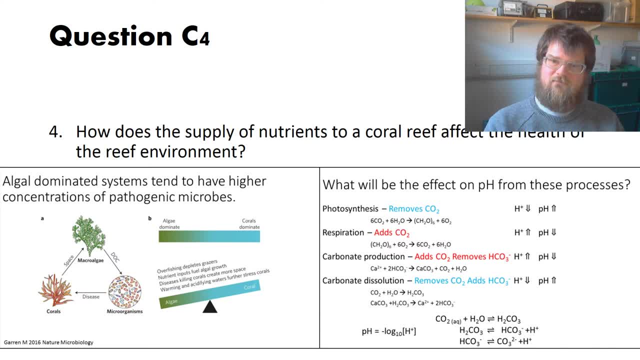 And that higher rate of biological production leaves more organic material in the water, which means that there's a potential for more pathogens in the water, more bacteria and viruses, So there's a mechanism by which there's an indirect control on the amount of disease in corals. 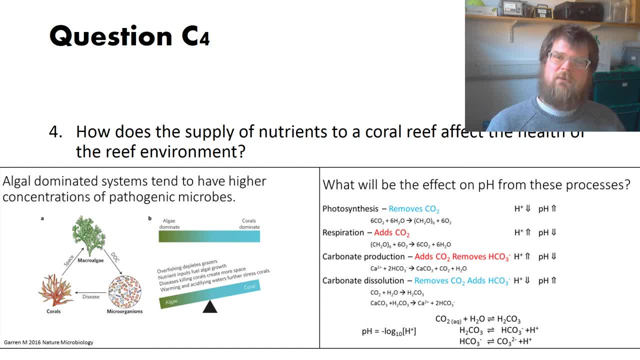 So quite a lot of you mentioned that. Most people that mentioned it didn't explain the link. As soon as I say nutrients equals more disease, Great, But they didn't explain that It's one of the Mechanisms is increased dissolved organic carbon leads to a higher pathogen load in the water, which can promote more disease. 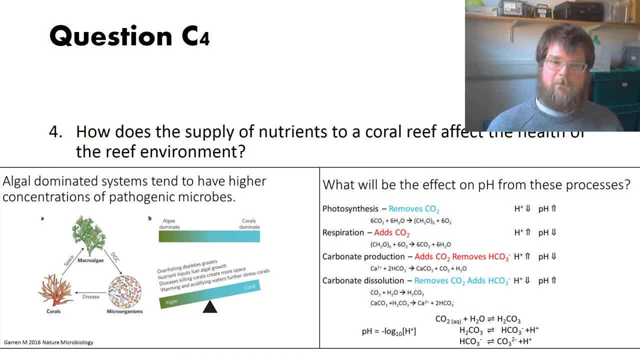 So it's that addition of the mechanism which would have given more mugs. Very few people mentioned the effect of nutrients on the pH of the of the reef environment. Now, this is very much an indirect effect because adding or taking away nutrients themselves in the water doesn't have a very large effect on the pH of the ocean, has a very small effect. 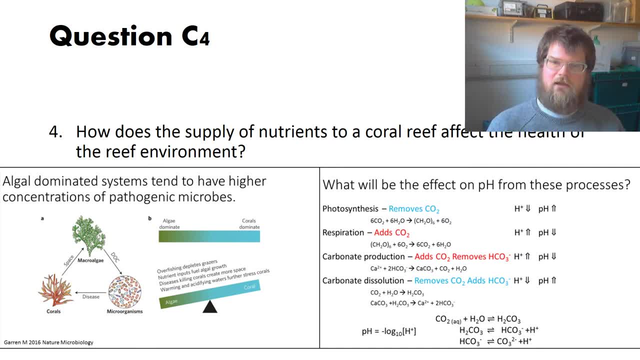 But the main drivers of pH change in the reef environment are these things here. So photosynthesis, photosynthesis and respiration, carbonate production and dissolution. Now, if you change the ecosystem by basically promoting algal growth, that means you might get more photosynthesis and maybe more respiration. So you might have a larger day night cycle of pH because you're having more photosynthesis, more respiration going on on a daily cycle. so that might give you larger swings in ph but it might not change the overall average ph because if you do more photosynthesis and more respiration 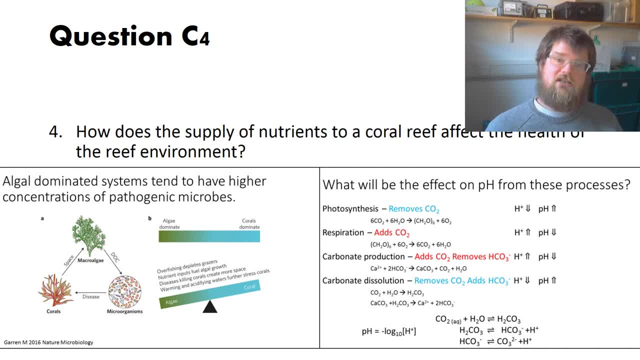 they kind of cancel each other out. um, but if you do change the ecosystem so that you have fewer corals, fewer carbonate producers, that means you'll be doing less of this. um, we got less of this carbonate production, and that carbonate production is actually acidifying the water, so there's a 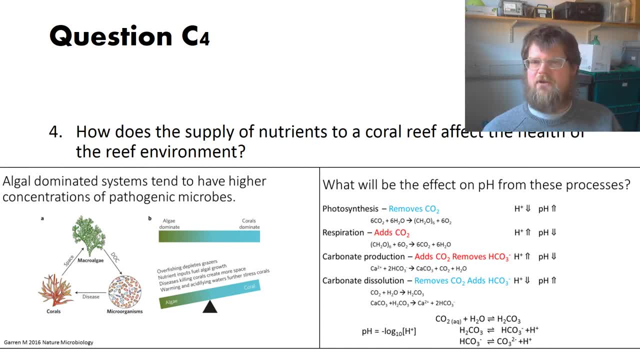 potential for a negative feedback here. so that's not negative because it's bad, but negative because it it might- um uh basically counteract the initial change. so if you have a um uh increase in nutrients, you might promote more algae, reduce the amount of coral cover, but that would then mean that you'd 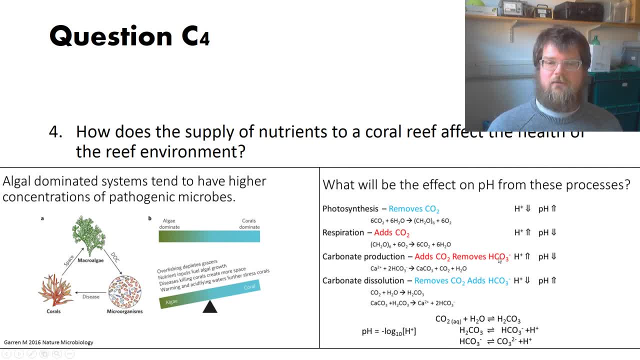 have less carbonate production, which would actually, um, uh, say less carbonate production. so if you have less carbonate production, then you're not doing this, and carbonate production acidifies the water. so if you have less of that, then you're going to effectively acidify the water less, so the ph will go up, uh, which then might make it more favorable for carbonate producers to kind. 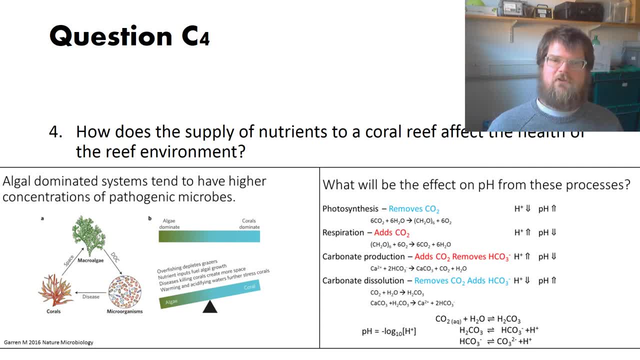 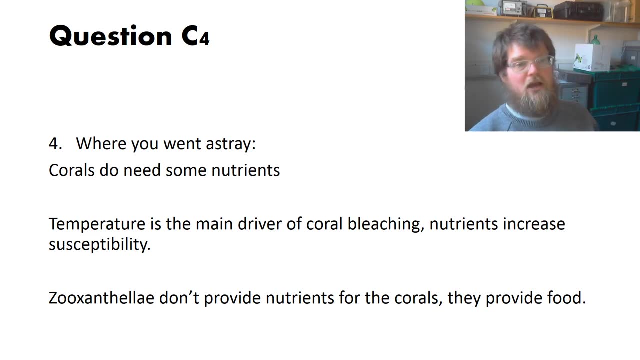 of be able to produce their skeletons or shells, um, so that might act to counteract the negative effect. i won't say i won't say negatively, uh, disadvantageous because effects of of nutrients through a negative feedback, um, anyway, so, uh, some some um, uh some, just some minor things that people uh got a little bit wrong, um, but corals do. 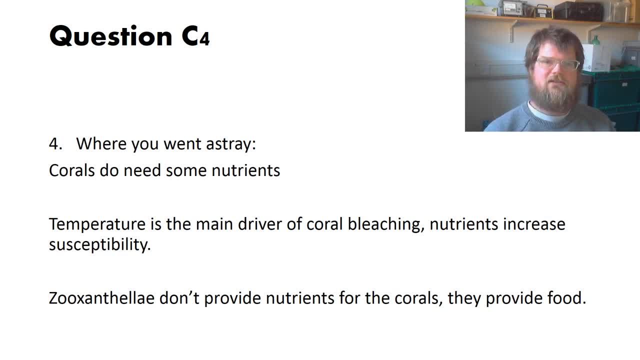 need some nutrients. um, so quite a lot of people missed out on that. uh, little nugget of wisdom there. so zero nutrients would be, you know, zero, zero activity. um, quite a lot of people um mentioned bleaching of corals. so this is when they eject the zooxanthellae and then become 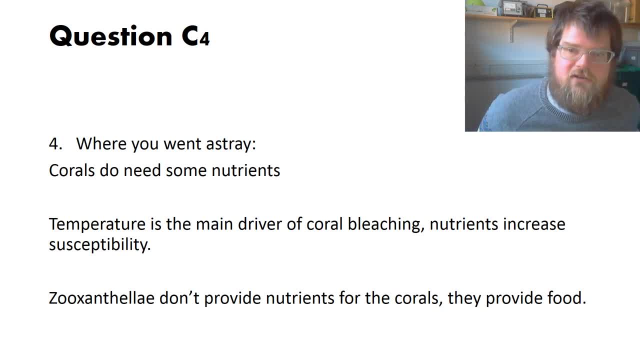 um, just filter feeders and are unable to photosynthesize. um now, most people didn't mention that the primary cause of coral bleaching is actually temperature and not nutrients. uh and um, so it's the temperature that's the primary cause of bleaching, and having a high nutrient loading might make the corals more susceptible to those. 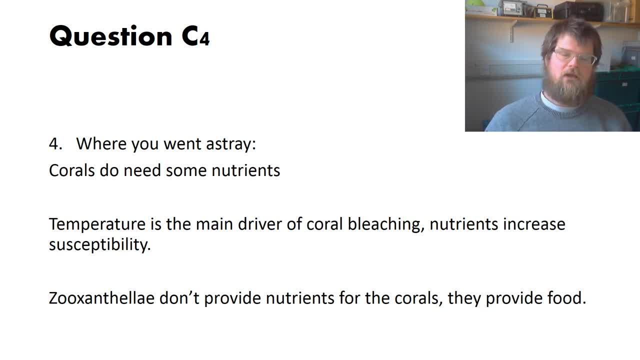 bleaching events but might not be the actual cause of them. um, it's very much like being um sunburned and having ginger hair. the ginger hair doesn't cause you to be sunburned, the sun causes you to be sunburned, but having, you know, paler skin does make you more susceptible. 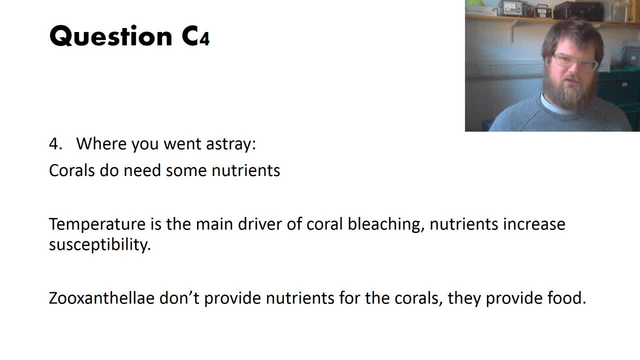 to sunburning. um, not a great analogy, but nonetheless um one that's vaguely correct. um, another thing: that people, um quite a few people, said that that the zooxanthellae provide nutrients for the corals, and i think this is a slight confusion between nutrients and food. 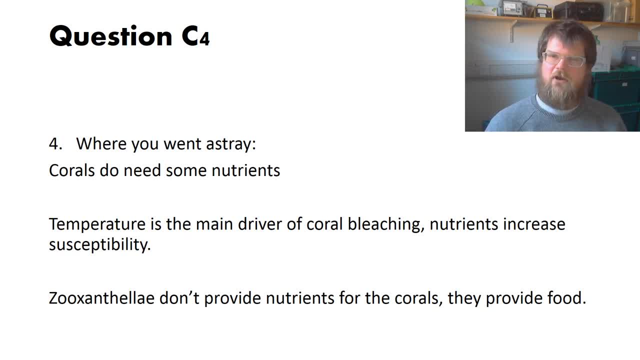 um, so i think it's a good thing that the zooxanthellae provide nutrients for the corals. i think, well, certainly when i'm eating, i might consider that i'm- when i'm eating food, i'm consuming nutrients, uh, which is kind of true, but for the corals, and particularly nitrogen phosphorus. 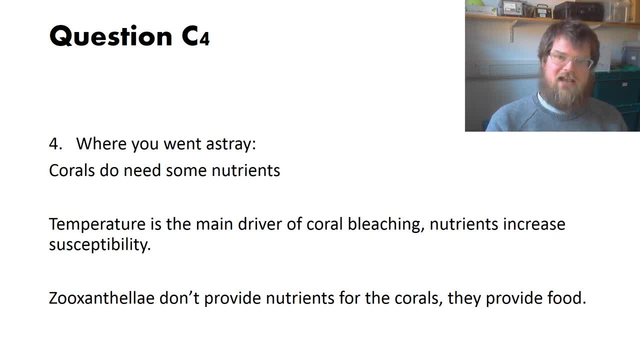 the, um, the corals actually supply the zooxanthellae with the nutrients and then the zooxanthellae the algae, they provide the corals with organic matter. so, um, the organic matter is not nutrient in this case. slight, uh, maybe semantics about what a nutrient is and whether 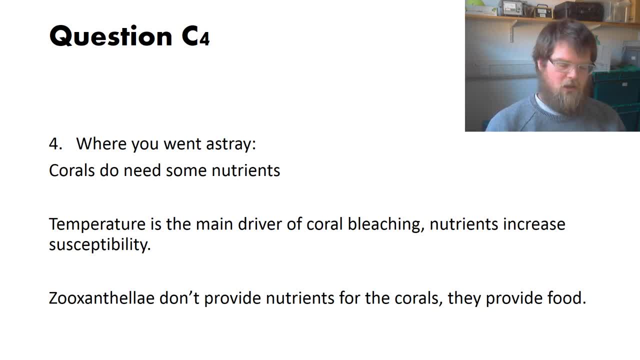 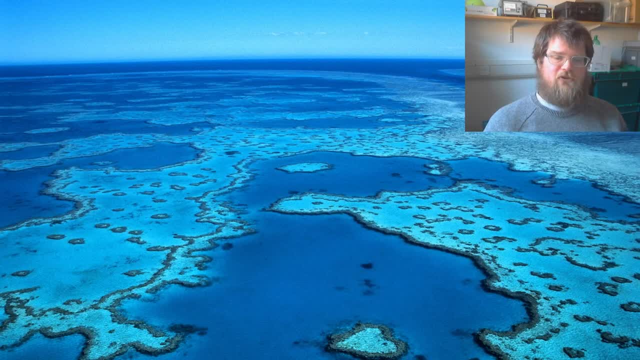 food is nutrient or not? um, but anyway, um, right, so, uh, so that's the end of uh that. that hopefully has um helped you find where, uh, what we were looking for in the the bulk of the exam questions. uh, maybe identified somewhere where you could have improved um, your um, your answers um, and, if you're 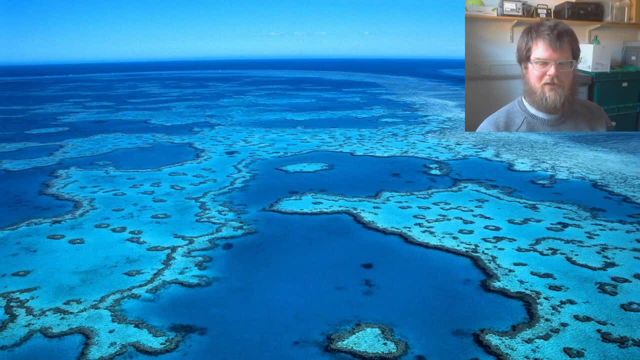 looking at this next year, in the future, through the medium time travel. um, then, uh, this is the kind of thing that you need to write in your exam question. um, so i think that's a good thing to write in your exam question, so do that. um, right, i'm gonna stop there using using the stop recording.